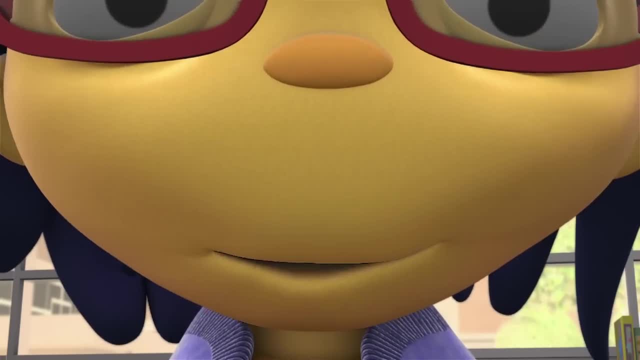 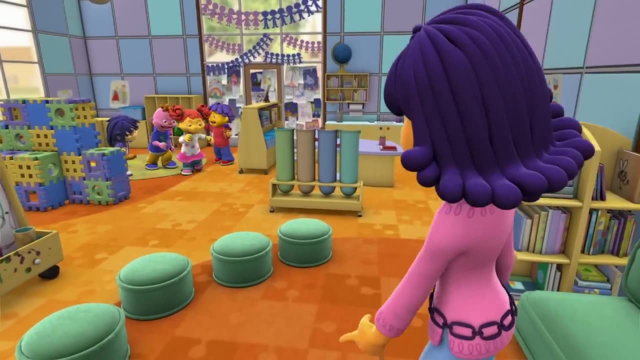 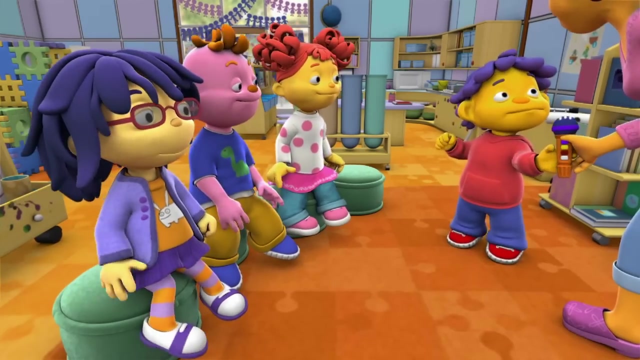 And now it's time for Susie to sing. Go, Susie. Wow, I heard your sound waves from all the way over here. You guys reminded me of a little song about the sound waves that we hear every day all around us. 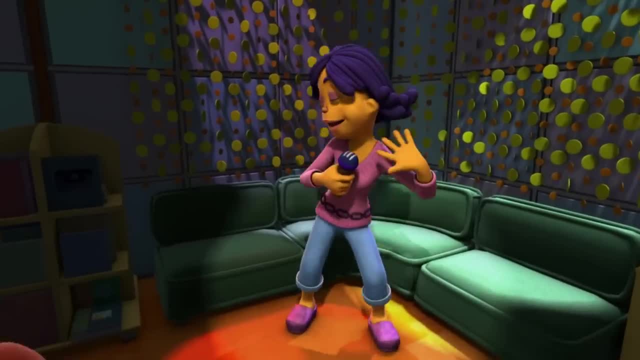 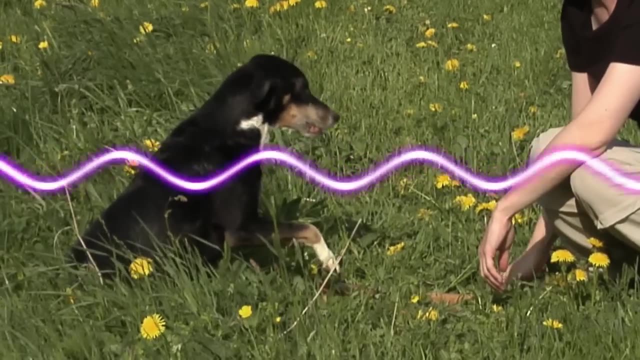 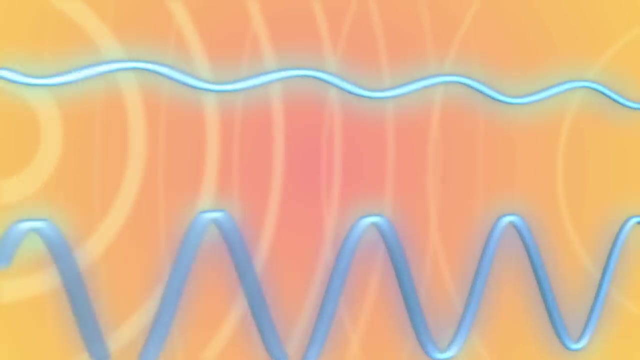 Waves of sound are riding through the air. Waves of sound for the world to hear. Take the time to listen to the sounds that you've been missing. Waves of sound bring music to my ears. Sound waves float in different lengths. Sound waves come in different strengths. 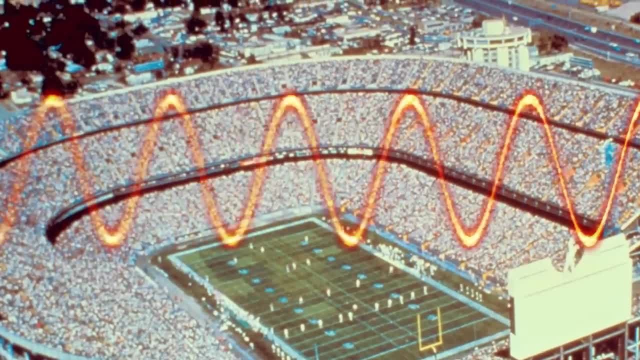 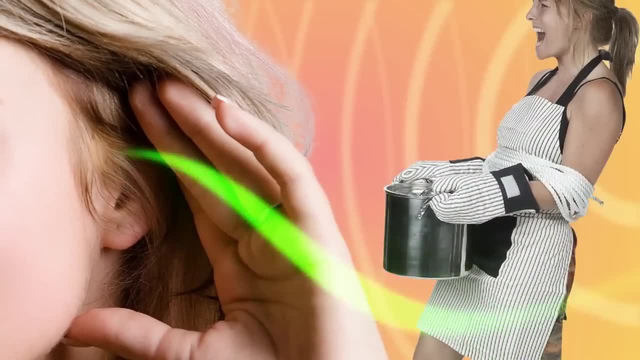 A tuba is big, so is a football crowd, A whisper is soft, a rocking band is loud, Your ears hear traffic and a song with rhyme, Mom calling you for tea Dinner. at the very same time, Some sounds are so loud you hold your ears when you're near them. 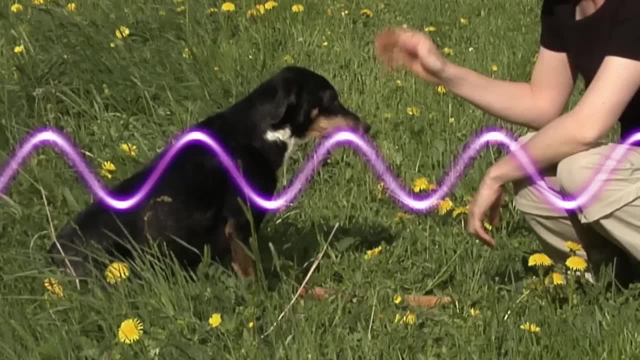 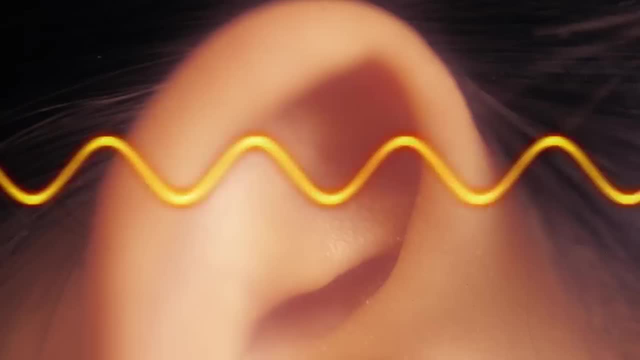 Some are so small you can barely hear them. Waves of sound are riding through the air. Waves of sound for the world to hear. Take the time to listen to the sounds that you've been missing. Waves of sound bring music to my ears. 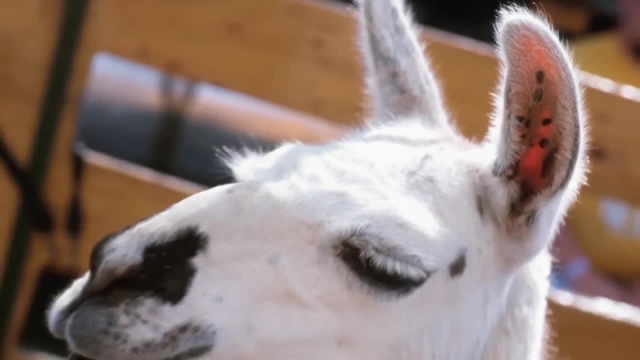 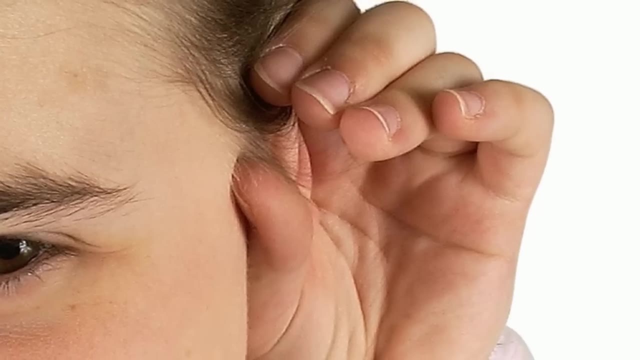 Ears are a natural listening tool. Some are long and sloppy, like the ears on a mule. You know a lot of animals have got a lot of ears. You can hear them too. You hear them and they hear. you Make a sound wave with your voice. 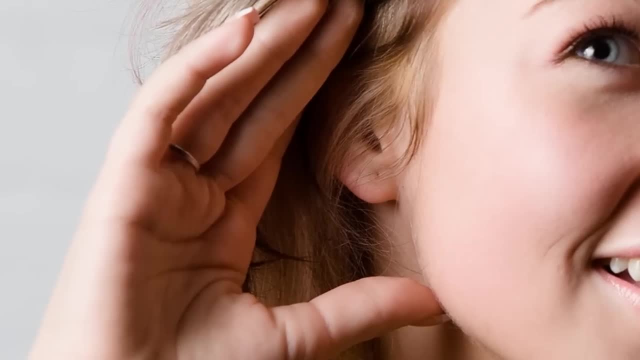 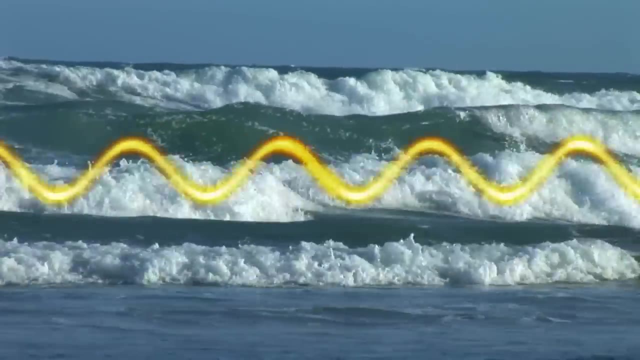 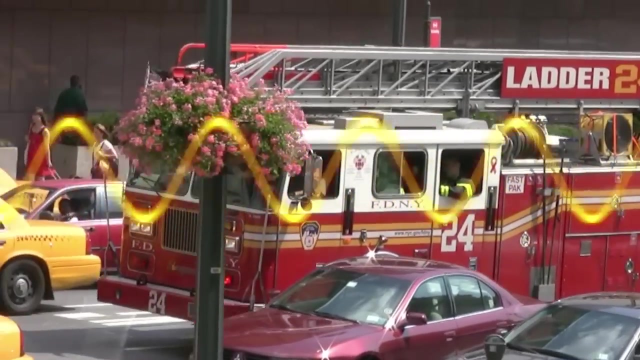 Make it loud or soft. now, that's your choice. Take the time to hear the sounds wherever you go. My favorite sound is a friend saying hello. Waves of sound are riding through the air, Waves of sound for the world to hear. Take the time to listen to the sounds that you've been missing. 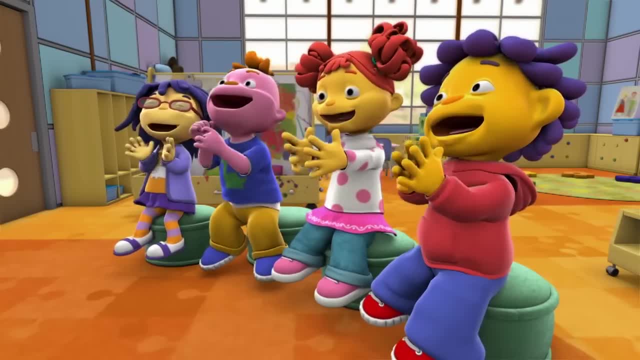 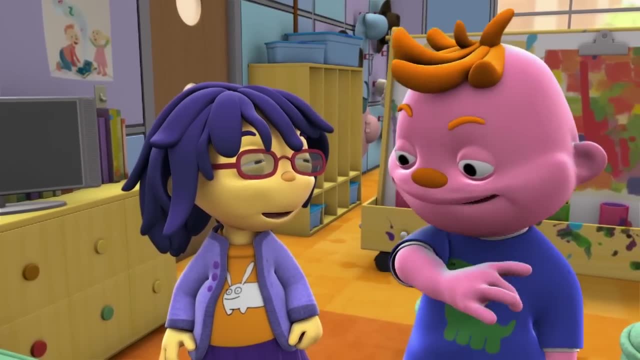 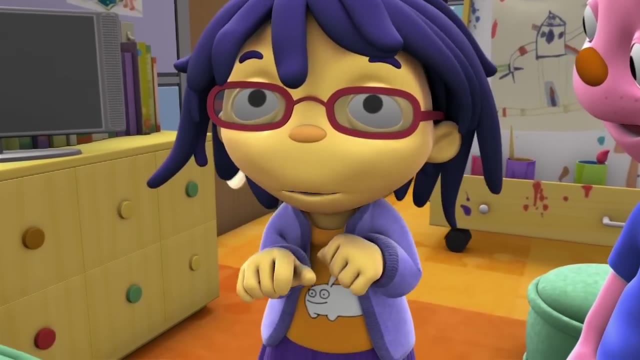 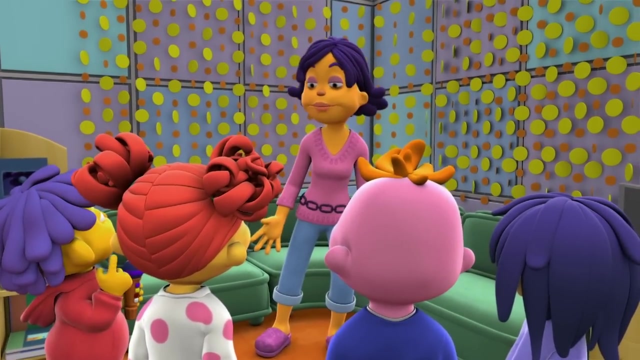 Waves of sound bring music to my ears. Yeah, So cool. I liked it in that song when the sound waves went through the air and into everyone's ears. I like it when you make little sounds and make little sound waves. Well, I'm using my sense of hearing to listen to my sound experts.